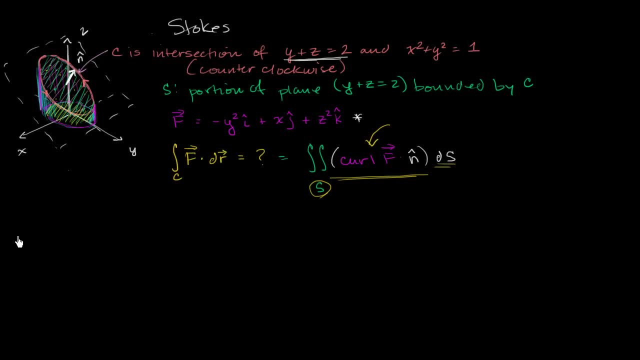 so it looks a little bit more traditional. So this is my x-axis, And then my y-axis would look something like that. Let me draw it a little bit different. This is my y-axis, And then if I were to draw the unit circle, 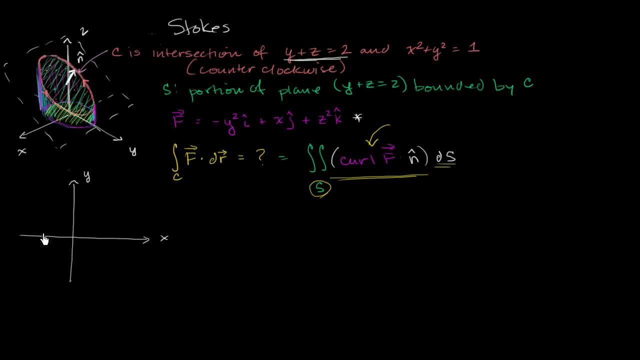 so kind of the base of this thing, or at least where it intersects the xy plane. Actually, this thing would keep going down if I wanted to draw: x squared plus y squared equals 1.. But if I draw where it intersects the xy plane, 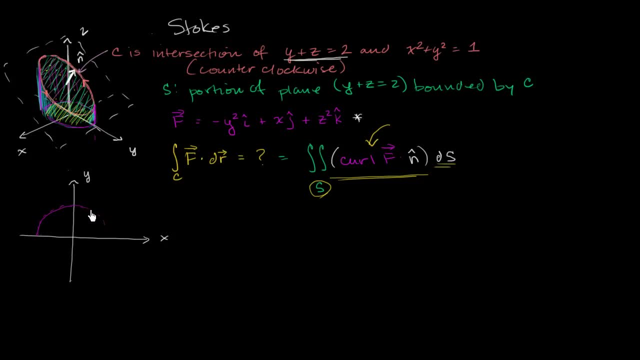 we get the unit circle, So let me just draw it. That's my best attempt at drawing a unit circle. We get the unit circle. We need to think of using parameters so that we can get every x and y coordinate. that's inside of the unit circle. 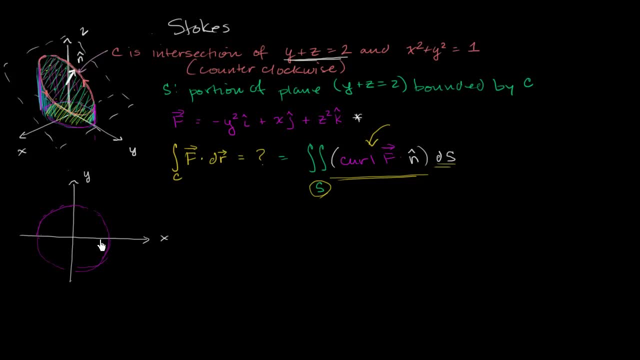 And to think about that, I'll introduce one parameter that's essentially the angle with the x-axis, And I'll call that parameter theta. So theta is the angle with the x-axis, And so theta will essentially sweep things all the way around. 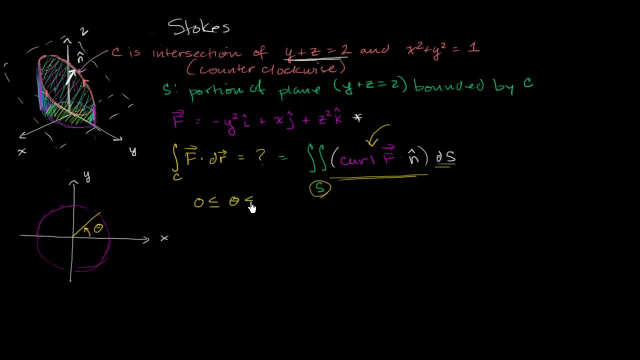 So theta can go between 0 and 2 pi. So theta will take on values between 0 and 2 pi. And if we just fix the radius at some point- say radius 1,, that would only give us all of the points on the unit circle. 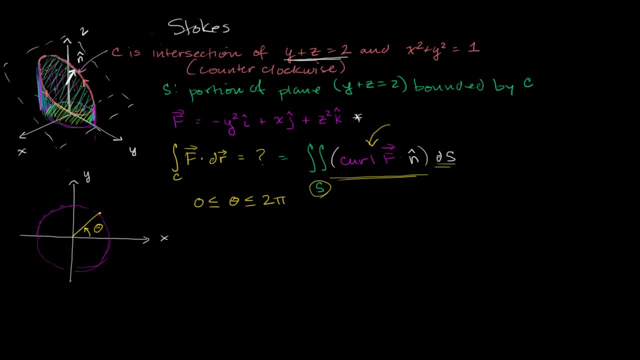 But we want all the points inside of it too, So we need to vary the radius as well. So let's introduce another parameter, Let's call it r, That is the radius. So for any given r, if we keep changing theta, 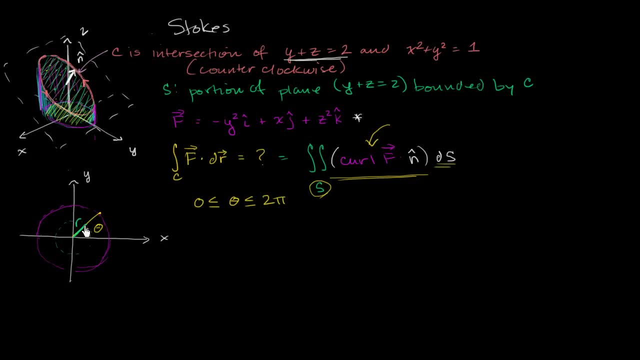 we would essentially sweep out a circle of that radius And if you change radius a little bit more you'll sweep out another circle, And if you vary radius between 0 and 1, you'll get all of the circles that will fill out. 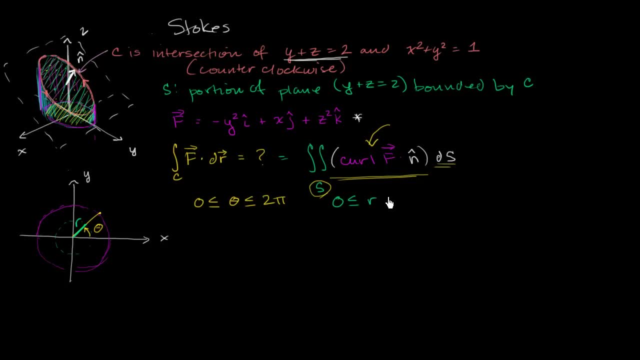 this entire area. So the radius is going to go between 0 and 1.. Another way of thinking about it is for any given theta, if you keep varying the radiuses, you'll sweep out all the points on this line And then, as you change theta, it'll. 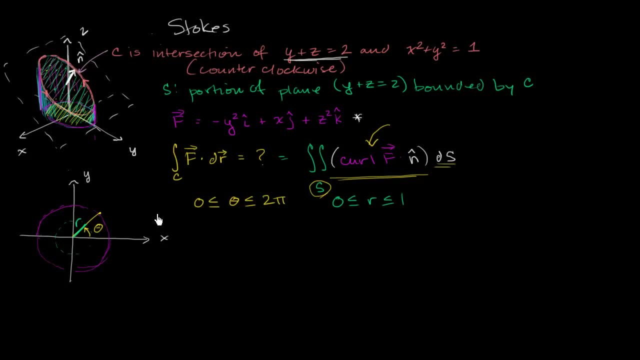 sweep out the entire circle, So either way you think about it. So with that let's actually define x and y in those terms. So we could say that x is going to be equal to So the x value. whatever r is the x value. 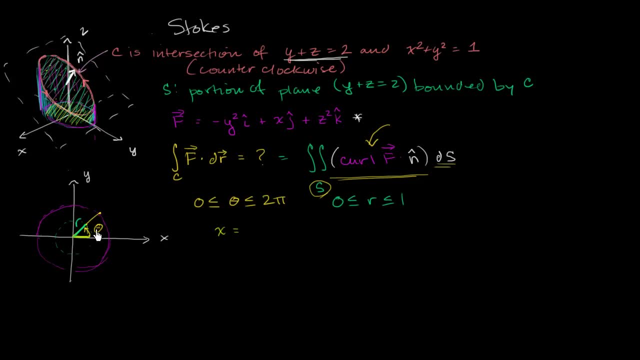 is going to be r cosine theta. It's going to be that component. It's going to be r cosine theta And then the y component- this is just basic trigonometry- is going to be the y, It's just going to be r.